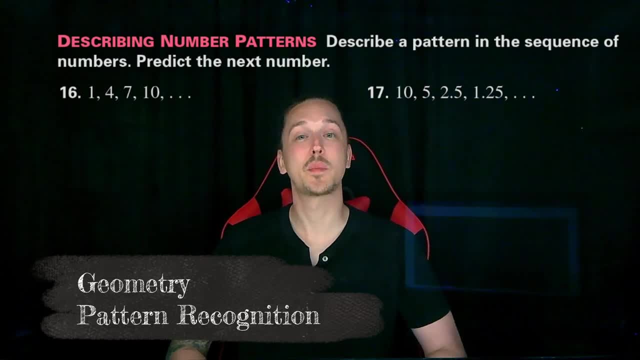 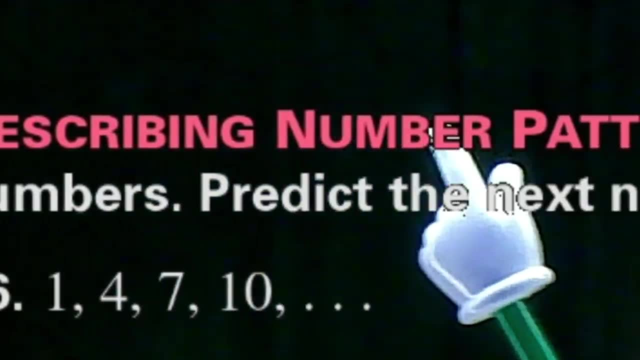 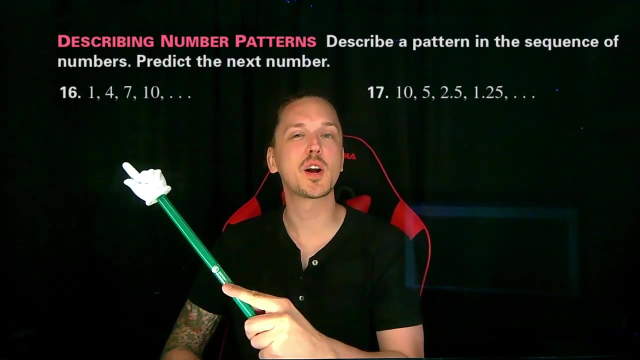 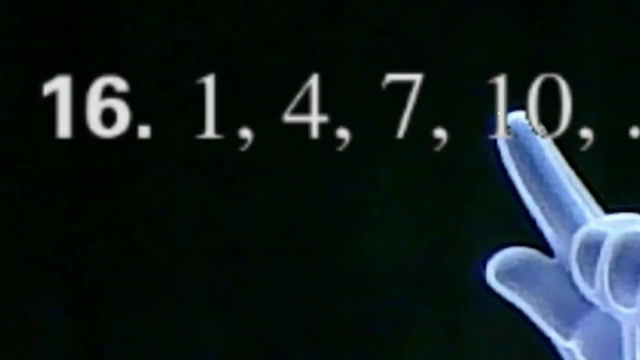 problem is a great introduction into basic geometric concepts such as pattern recognition. So let's unravel the mysteries together. First let's read the problem's instructions Describing number patterns. Describe a pattern in the sequence of numbers and predict the next number. Let's start here with number 16.. The numbers go from 1 to 4 to 7 to 10.. Do you see the? 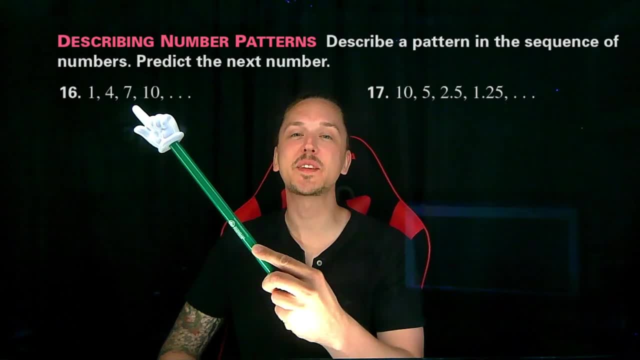 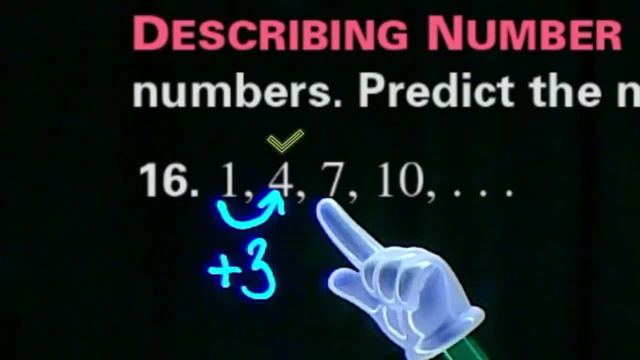 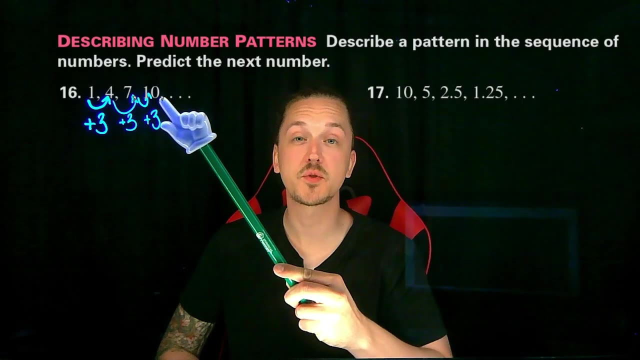 pattern here. Hey, if you said the numbers are going up by 3, you'd be correct. 1 plus 3 is 4, plus 3 is 7, plus 3 is 10.. So from 10, we would add 3. 10,. 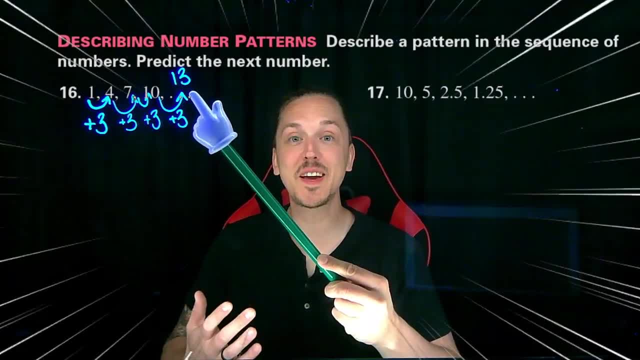 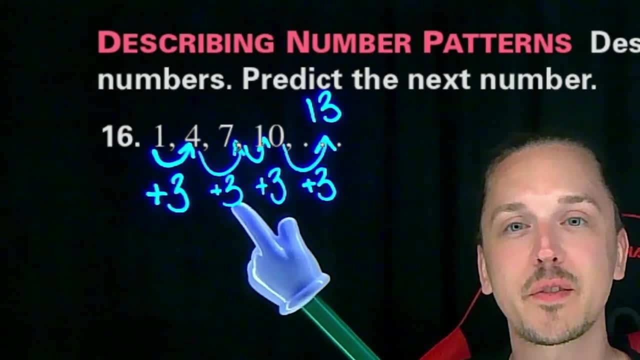 11,, 12,, 13.. 13! Yeah, 13 is the next number in our sequence, where our pattern is plus 3.. Hey, nice work. What do you say? we use that same thought process on number 17 here. 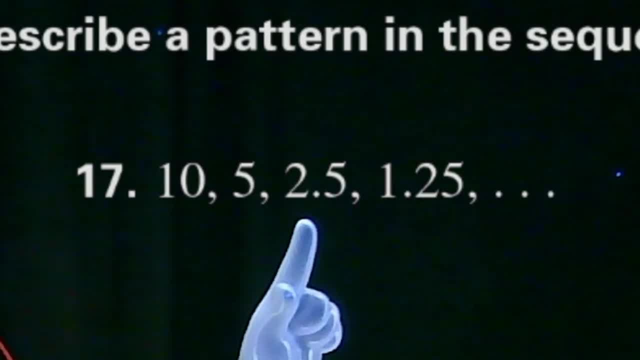 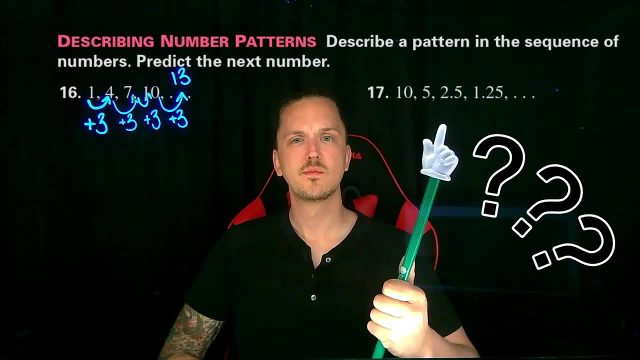 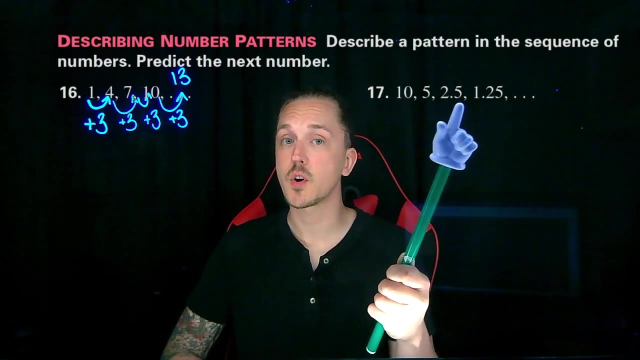 10 to 5 to 2.5 to 1.25.. What is the pattern here? Do you see the pattern? Do you see the last pattern, which went up by 3? each time This pattern's numbers are going down. 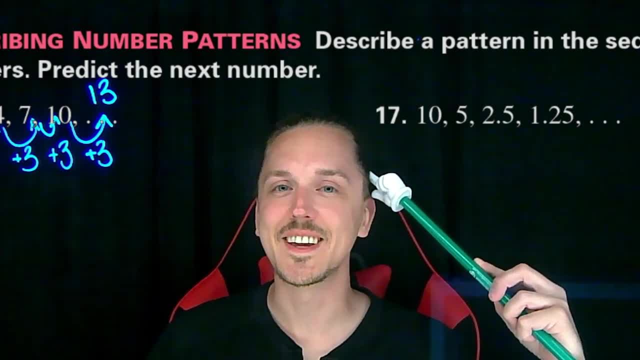 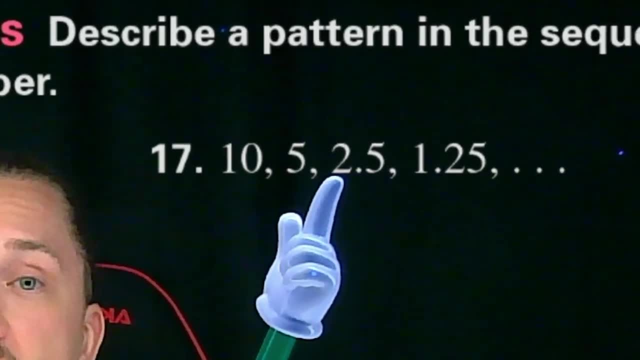 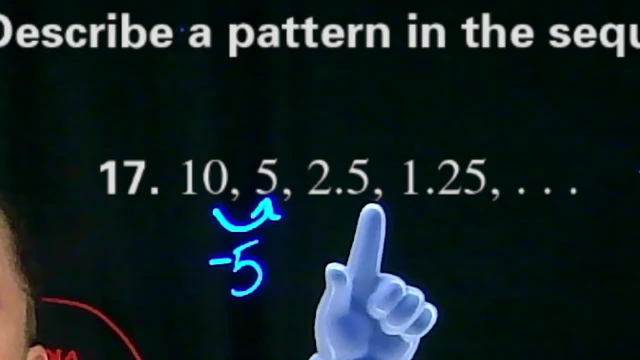 So you might check subtraction. Let's see: Going down from 10 to 5 is a subtraction of 5, or minus 5.. And going down from 5 to 2.5 is also a subtraction of 2.5, or minus 2.5.. Then going down from 2.5 to 1.25 is also a subtraction of 2.5, or minus 2.5.. 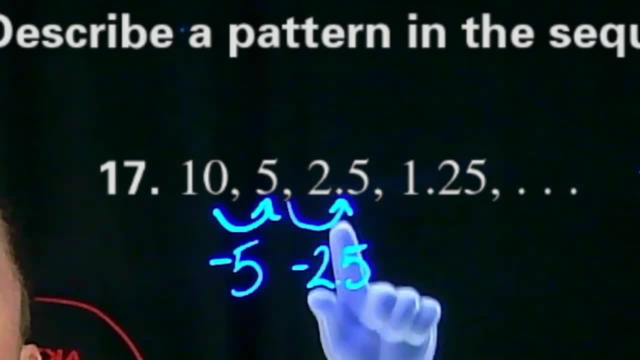 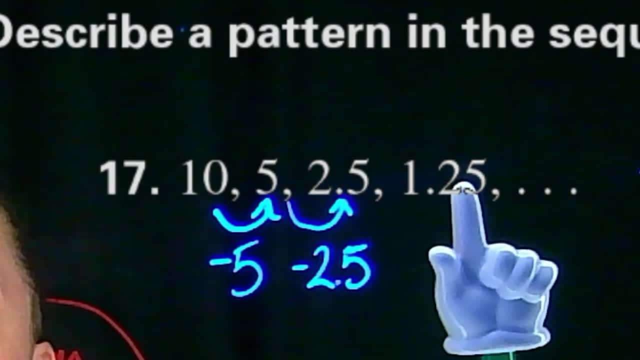 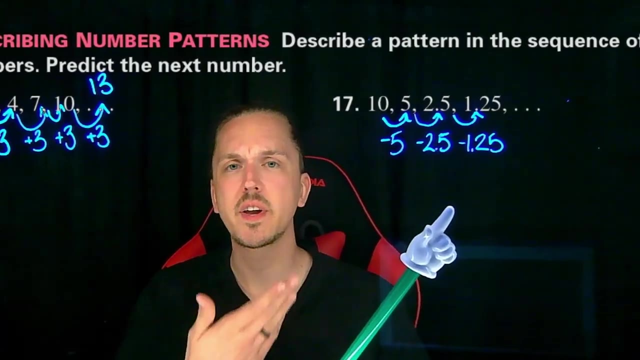 Then going down from 2.5 to 1.25 is also a subtraction of 1.25, or minus 1.25.. Interesting, But this seems a little complicated compared to our previous one. Maybe there's another way that we can approach this pattern that doesn't involve subtraction. 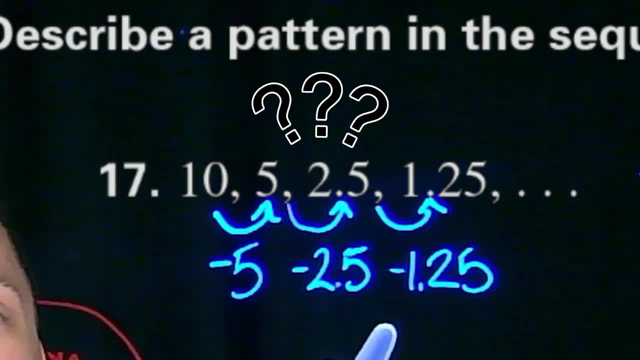 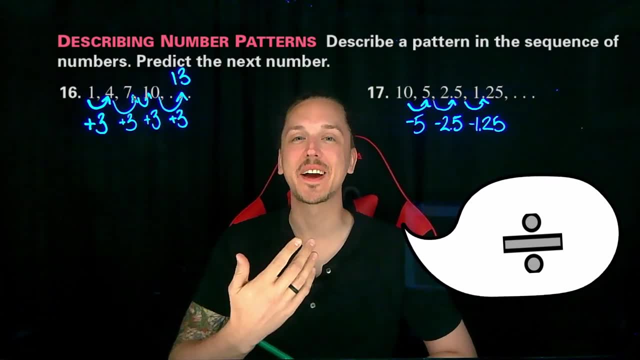 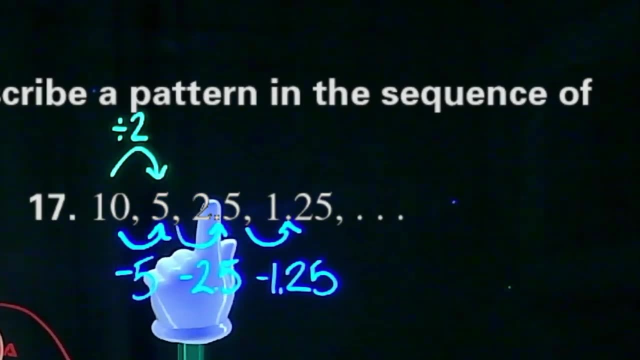 Do you see another way that we can describe this pattern that doesn't involve subtraction? Yeah, what about division? Division can be used to make a number smaller. Let's try it. To go from 10 to 5, we will divide by 2.. To go from 5 to 2.5, we will also divide by 2..